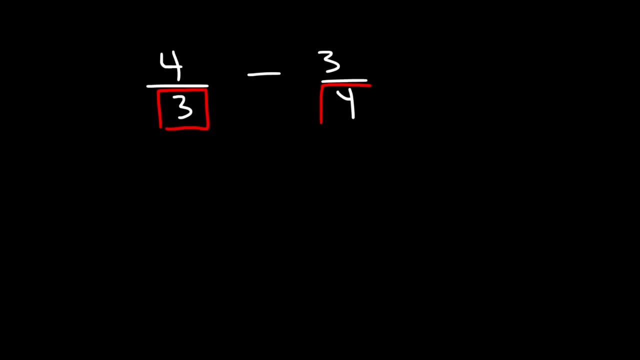 So first let's multiply the two denominators of the fractions: 3 times 4 is 12.. And then cross multiply: 4 times 4 is 16.. 3 times negative, 3 is negative 9.. Now 16 minus 9 is 7.. 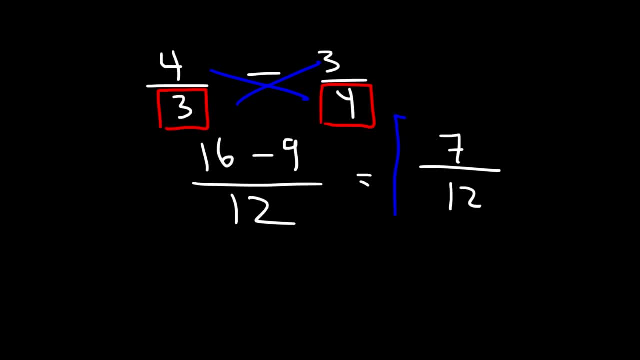 So the answer is going to be 7.. So now it's your turn. Go ahead and subtract these two fractions: 3 over 8 minus 1 over 7.. And also 5 over 7 minus 2 over 5.. 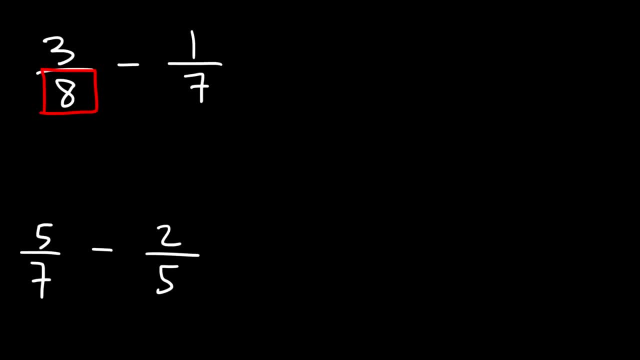 So, starting with the first example, let's multiply 8 by 7.. So 8 times 7 is 56. And then let's cross: multiply 3 times 7 is 21.. And 8 times negative 1 is negative 8.. 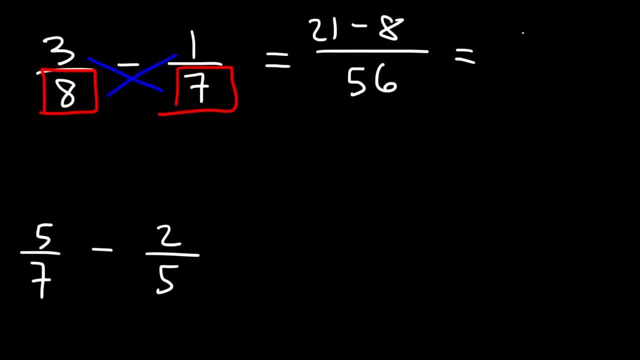 So now we need to subtract: 21 minus 8 is 13.. So the answer to the first problem is going to be 13 over 56.. Now for the next example. let's multiply 7 and 5.. 7 times 5 is 35.. 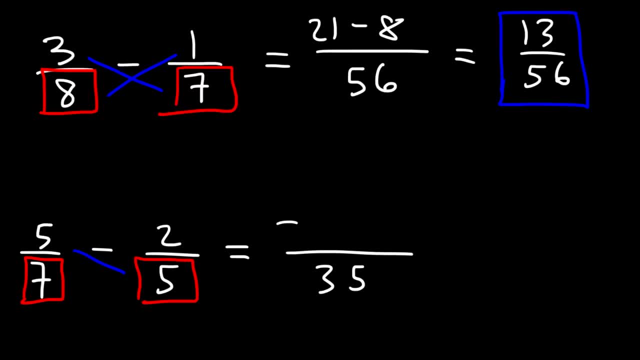 5 times 5 is 25.. And then we have 7 times 2, which is 14.. So now let's subtract 25 and 14.. 25 minus 14 is 11.. And so this is going to be 11 over 35.. 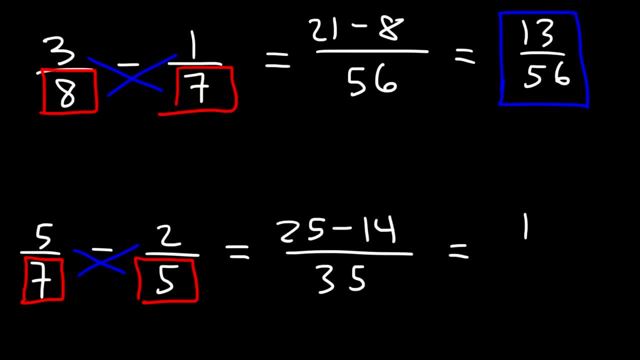 By the way, I'm going to post some links in the description section of this video where you can find more of my videos on fractions, like how to multiply fractions, like how to multiply fractions, how to multiply fractions, how to multiply fractions. 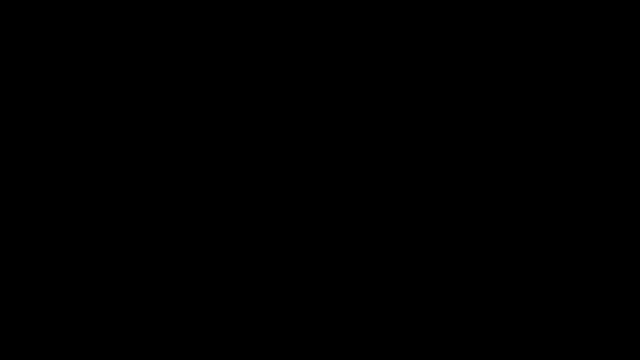 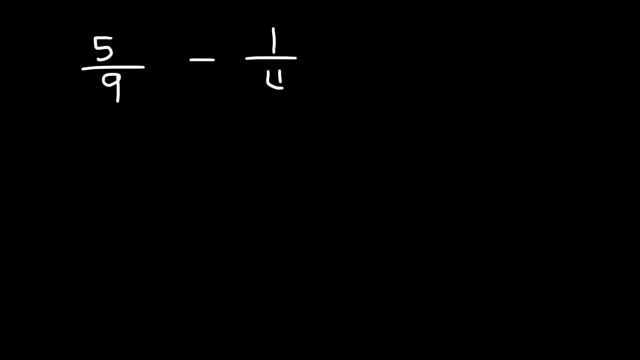 in which we can subtract 2 fractions. So in the previous method we would multiply 9 and 4.. And that will give us 36. And then we would cross: multiply 5 times 4 is 20.. And then 9 times 1 is 9.. 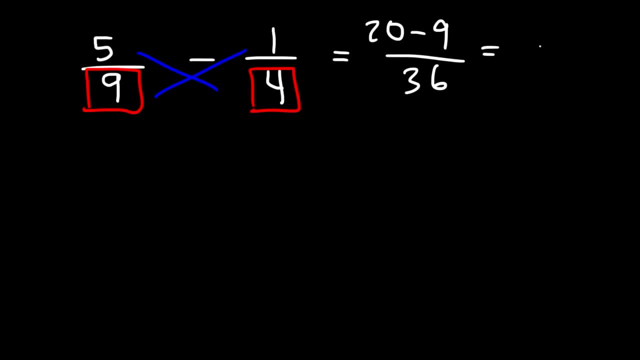 And then 9 times 1 is 9.. 9 times 1 is negative 9.. So it's going to be 20 minus 9,, which is 11.. And so this will give us 11 over 36.. And so this will give us 11 over 36.. 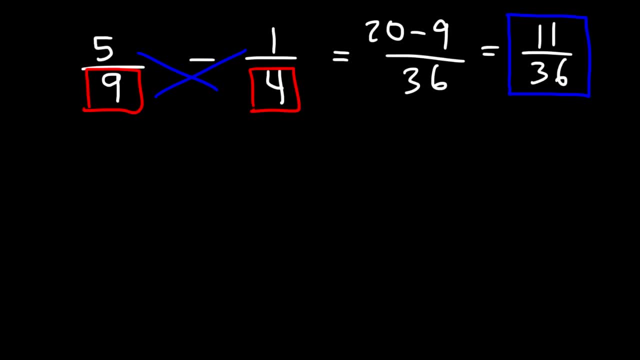 Now, another way in which you can do the same problem and get the same results is to get the common denominators first. before combining the 2 fractions, 9 times 4 is 36.. So to get a common denominator of 36,. 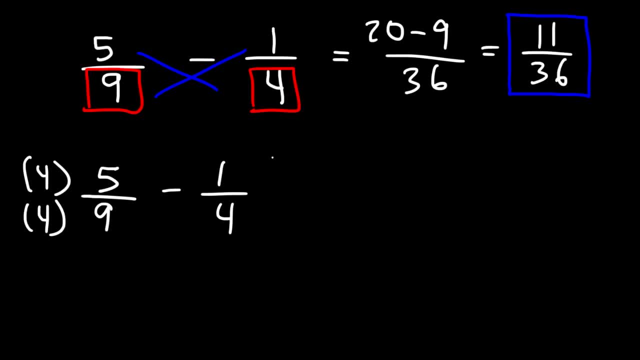 we need to multiply the first fraction by 4 over 4, and the second one by 9 over 9.. 4 times 5 is 20.. 4 times 9 is 36.. And so we're going to get this. 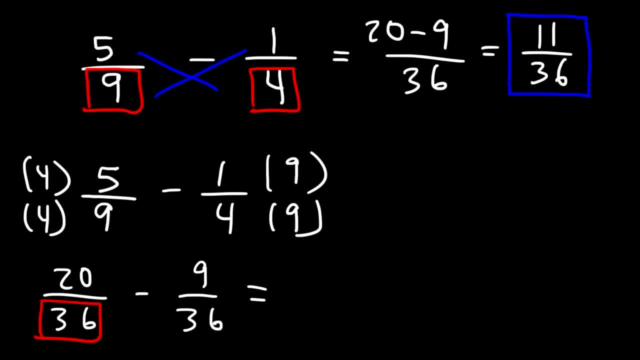 So now that these 2 are the same, we can combine the numerators of the 2 fractions. So 20 minus 9 is 11.. And so we're going to get the same answer: 11 over 36.. Now this technique is: 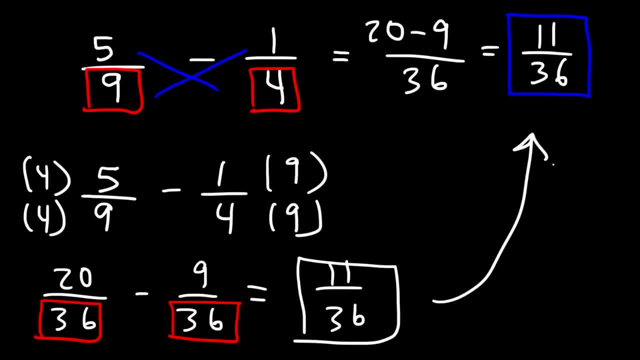 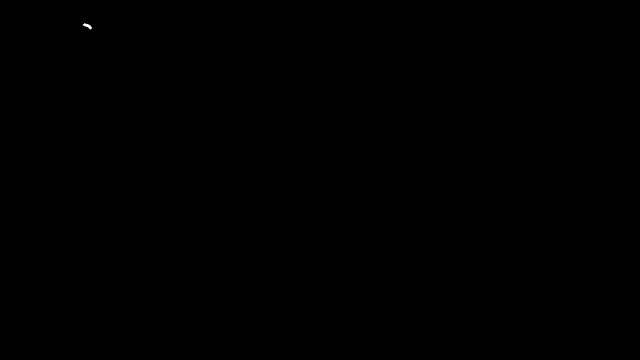 useful if you have multiple fractions. Let's say, if you want to subtract 3 or 4 fractions, You could do that. So let's say, if we have 8 over 9, minus 1 over 3, minus 2 over 5.. 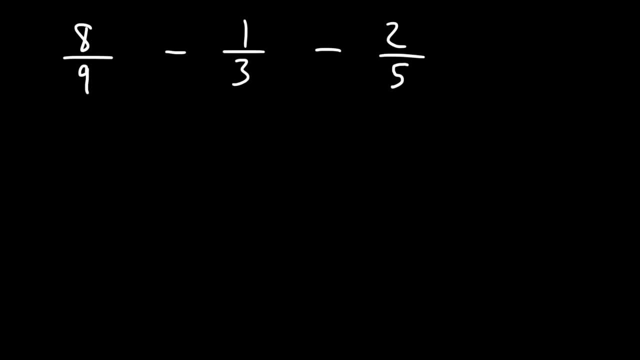 So we'll need to find a common denominator of those 3 fractions. So what is the least common multiple of 9,, 3, and 5?? 3 already goes into 9.. So any multiple of 9 is a multiple of 3.. So we don't really. 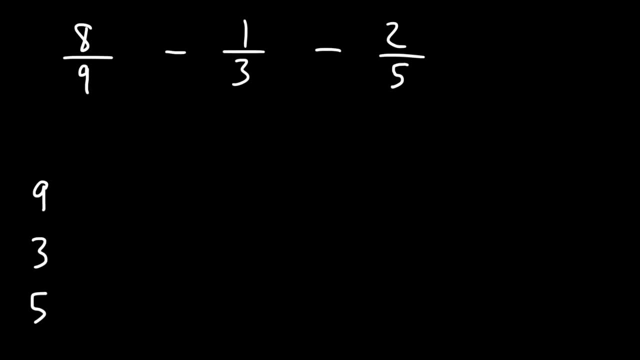 need to worry about this. So what is the common multiple between 9 and 5?? Well, 9 times 5 is 45. So 45 is the lowest number that can go into 9,, 3, and 5.. 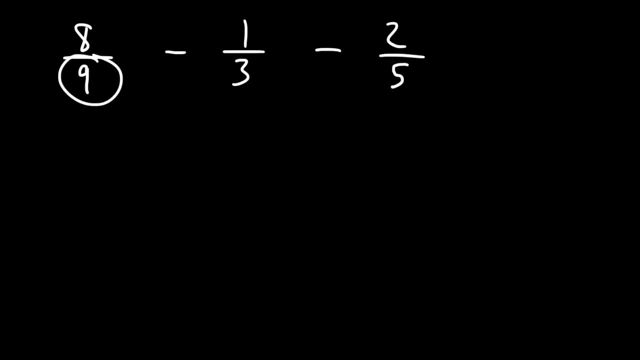 Now, 45 divided by 9 is 5.. So I'm going to multiply this fraction by 5 over 5.. Now, 45 divided by 3 is 15.. So I'm going to multiply the second fraction by 15. 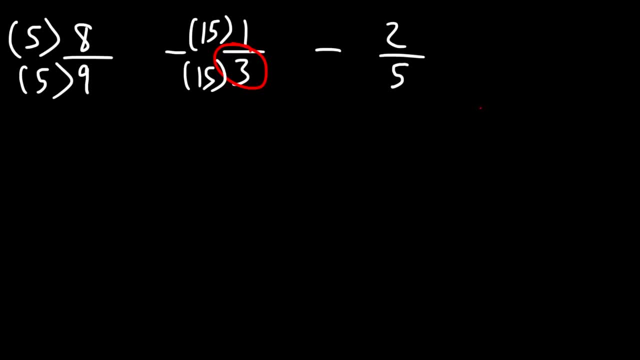 over 15.. And 45 divided by 5 is 9.. So I'm going to multiply the last fraction by 9 over 9.. 5 times 8 is 40.. 5 times 9 is 45.. 15 times 1 is 15.. 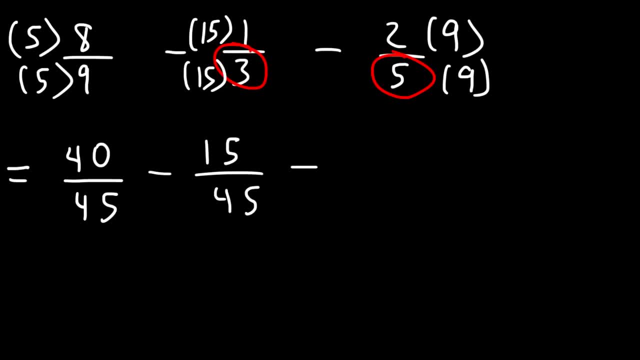 15 times 3 is 45.. 2 times 9 is 8.. 18.. 5 times 9 is 45.. And now we need to subtract. So 40 minus 15 is 25.. And 25 minus. 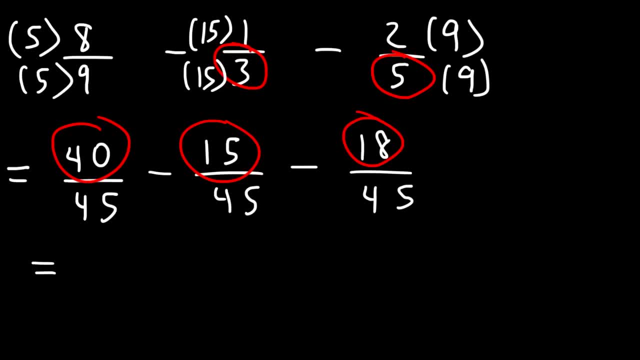 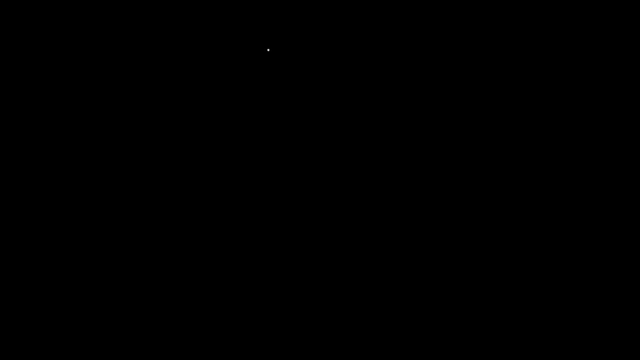 18 is 7.. So this is going to be 7 over 45. And that's the answer. Let's try another example: 9 over 10 minus 1 over 5 minus 2 over 7.. Feel free to pause the video and work on that example. 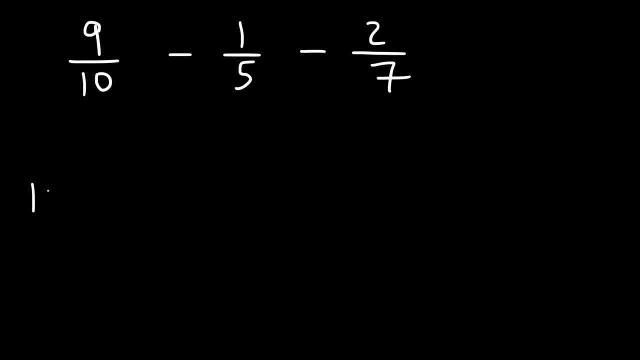 So let's get a common denominator between 10,, 5, and 7.. So 5 goes into 10.. So we don't have to worry about the 5.. Any multiple of 10 is going to be a multiple of 5.. 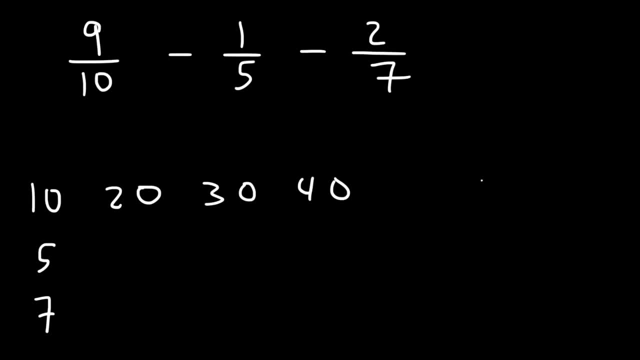 So multiples of 10 are 10,, 20,, 30,, 40,, all the way to 70.. 7 or 7,, 14,, 21,, 28,, all the way to 70.. If you multiply 10 and 7,, 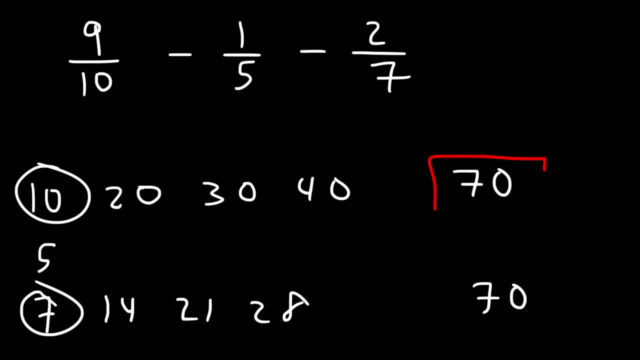 you're going to get a common multiple between 10 and 7, which is 70.. So it turns out that 70 is the common denominator that we want to get to. 70 divided by 10 is 7.. So let's multiply the first fraction. 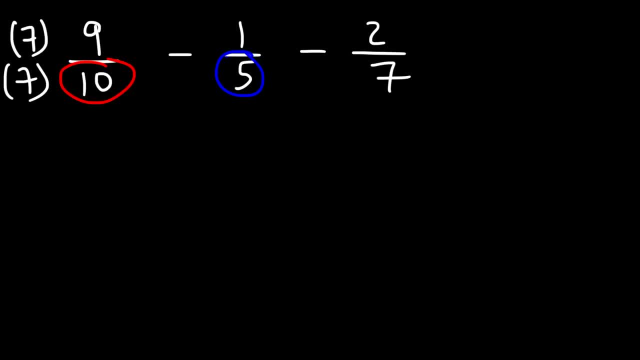 by 7 over 7.. 70 divided by 5- Let's see what that is. So let's use long division. 5 goes into 7 one time. 5 times 1 is 5.. And then subtract: 7 minus 5 is 2.. 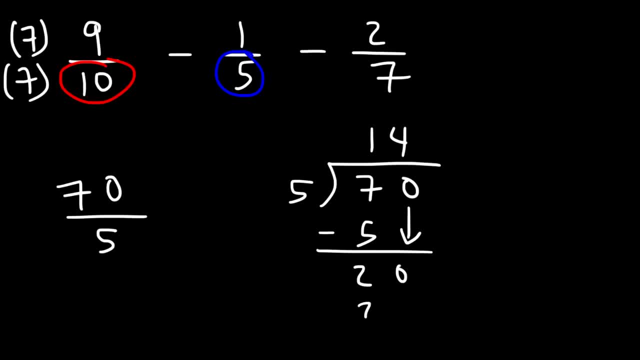 Bring 9 to 0.. 5 goes into 20 four times. So 70 divided by 5 is 14.. So we need to multiply this fraction by 14 over 14.. 70 divided by 7 is 10.. 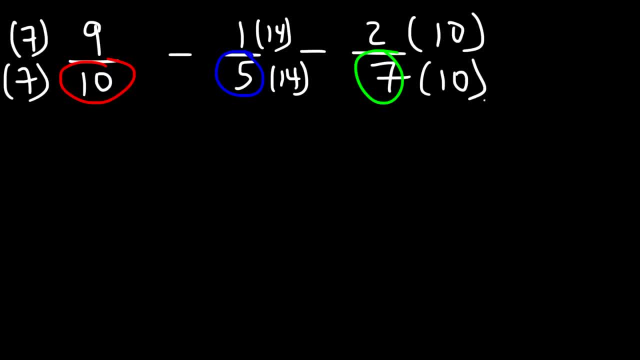 So we're going to multiply the last fraction by 10 over 10.. 7 times 9 is 63. And we know, 7 times 10 is 70. And 5 times 14 is 70. And 2 times 10 is 20.. 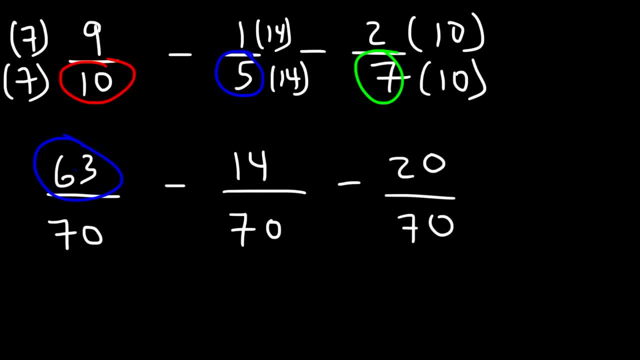 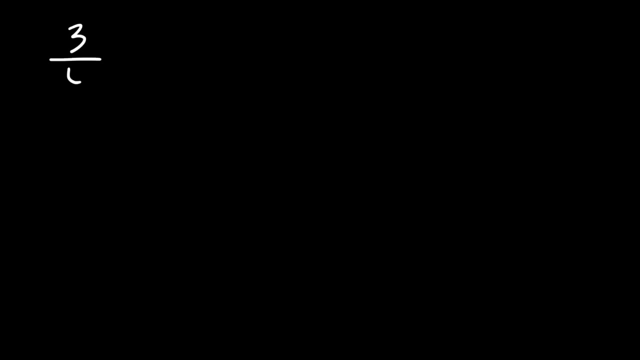 So now let's subtract 63 minus 14, That's 49.. And 49 minus 20 is 29.. So the final answer for this problem is 29 divided by 70.. Let's work on one last example: 3 over 4. 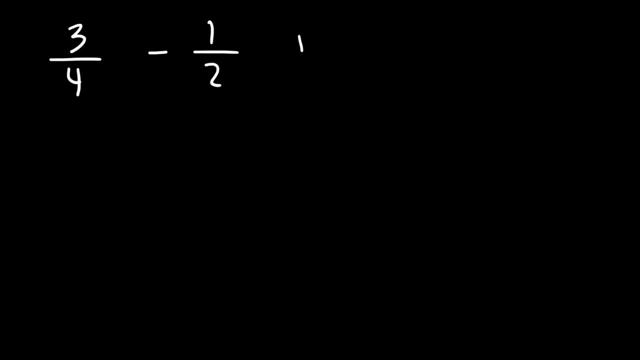 minus 1 over 2 plus 5 over 3, minus 2 over 5.. Go ahead and try that example. So what is a common multiple between 2,, 3,, 4, and 5?? Well, we don't have to worry about the 2, because 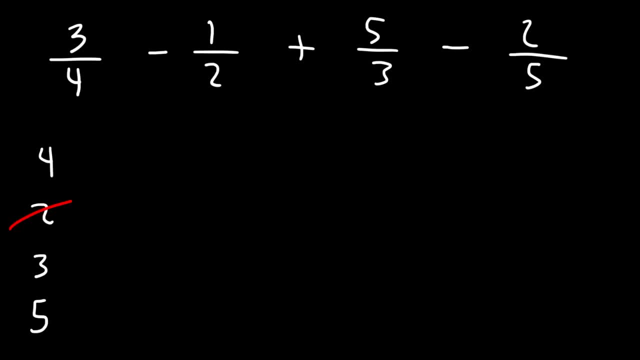 2 goes into 4.. So all we need to do is multiply 4 times 3 times 5,, which is 60. And so 60 is going to be the common denominator that we need to get to 60 divided by 4. 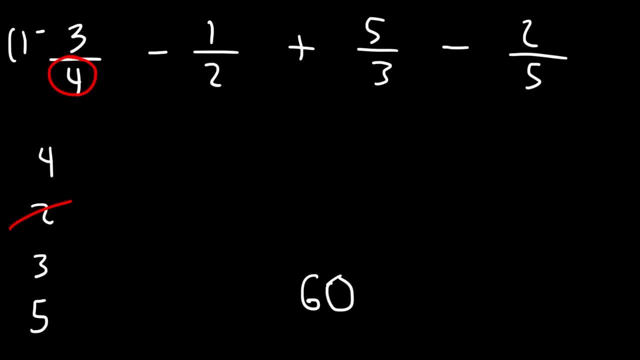 is 15.. So we're going to multiply this fraction by 15 over 15.. 60 divided by 2 is 30.. So we're going to multiply the second fraction by 30 over 30.. And 60 divided by 3. 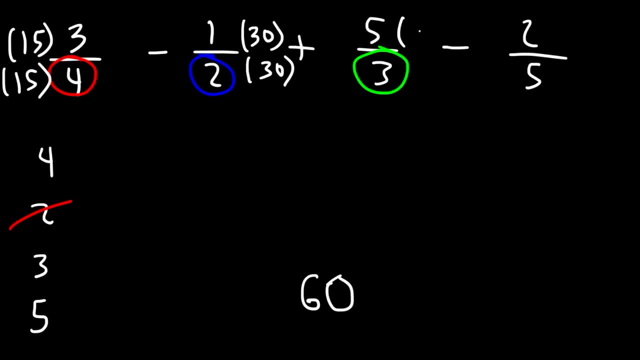 is 20.. So let's multiply this fraction by 20 over 20.. And finally, 60 divided by 5 is 20.. And 60 divided by 5 is 12.. Now let's multiply 15 times 3 is 45.. 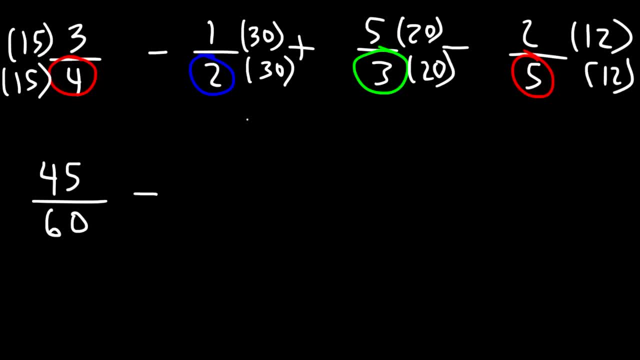 And we know: 15 times 4 is 60.. 1 times 30 is 30. And 2 times 30 is 60.. 5 times 20 is 100.. 3 times 20 is 60.. 2 times 12 is 24.. 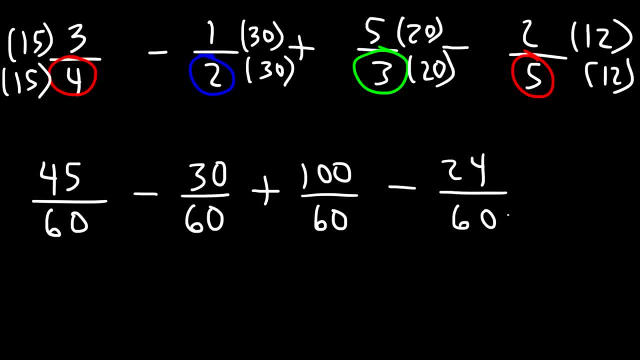 And 5 times 12 is 60. So now we'll need to subtract. So first let's subtract these two numbers: 45 minus 30 is 15.. So we have 15 over 60. And then let's subtract these two: 100 minus 24.. 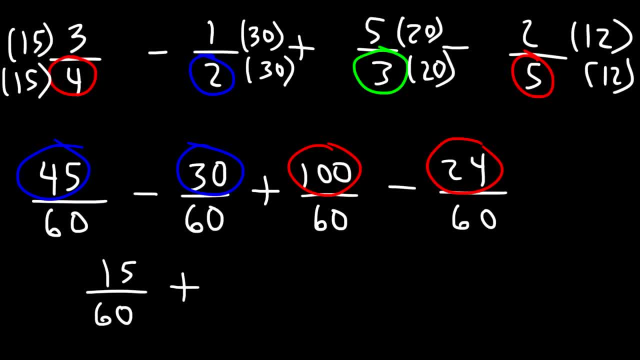 100 minus 20 is 80.. 80 minus 4 is 76.. So now we need to add 15 and 76.. 15 plus 76 is going to be 91. And so that is the final answer: It's 91 over 60.. 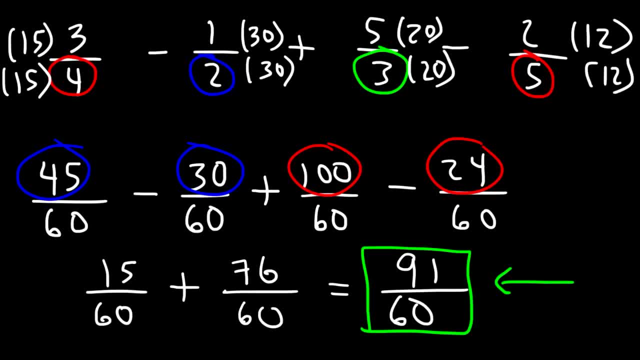 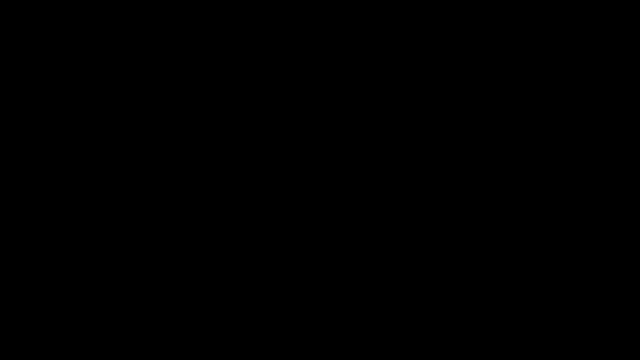 So that's all I got for this video. Be sure to check out my next video on multiplying fractions. Thanks for watching. I'll see you in the next one. Bye. 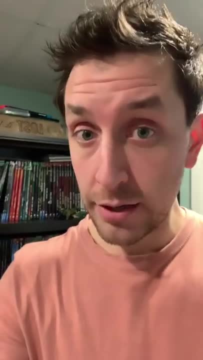 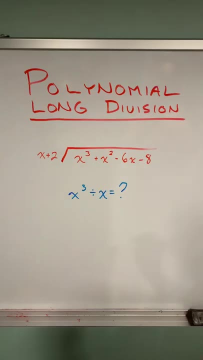 Want to do some polynomial subdivision. Neither do I, But you need the practice. So let's divide this expression by this binomial. So we set this problem up with our dividend here and our divisor on the left side, and we ask ourselves: how many times does this x go into this x cubed Well x. 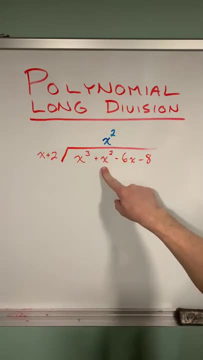 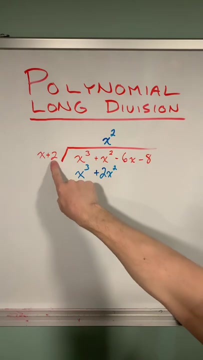 cubed divided by x is x squared and we're going to place that over top of this x squared. We're going to take that x squared and multiply by x and get x cubed and we'll place that directly below this x cubed. We'll take that same x squared and multiply it by this 2 to get 2x squared, placing: 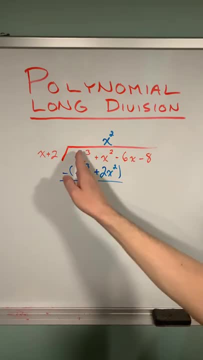 that below this x squared, We can place the result in brackets and subtract these two columns. That's going to result in negative x squared. We're going to bring this negative 6x down and repeat the whole process. Negative x squared divided by x is negative x, so I place that over. 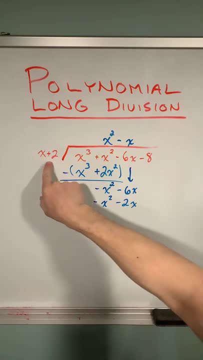 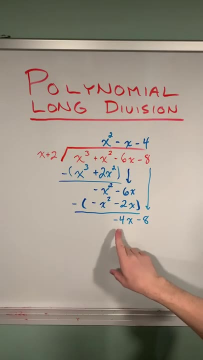 the x term in the dividend. I can multiply that negative x by each of these terms to produce this expression here and subtract straight down to get negative 4x and bring that negative 8 down and repeat the process to see that negative 4x divided by x is negative 4.. Multiplying negative: